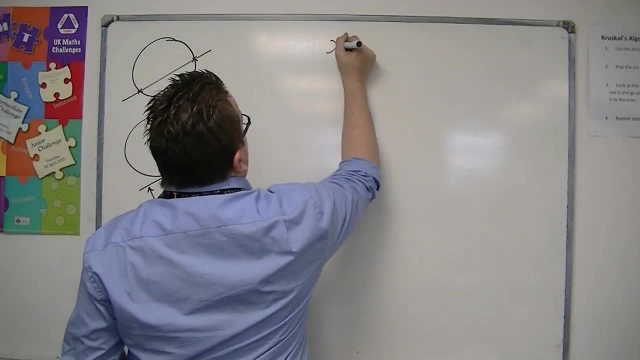 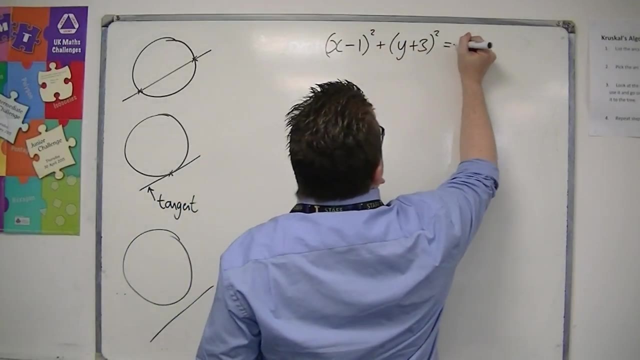 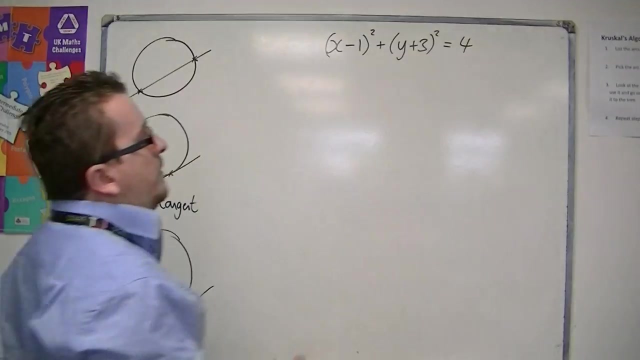 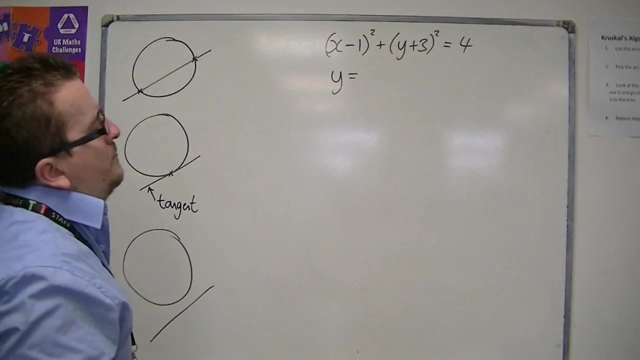 say We've got the circle x minus 1 squared plus y plus 3 squared is equal to: let's say: let's choose a nice number 4.. And then we have a straight line: y is equal to: let's have: 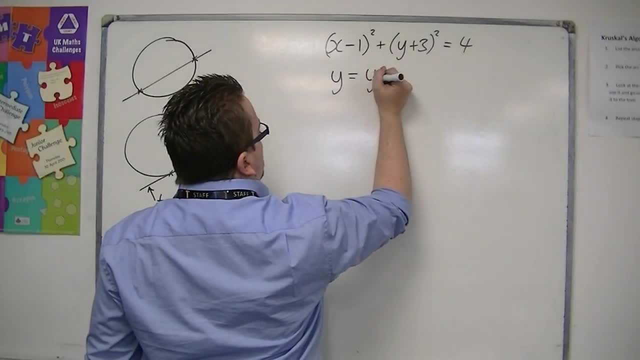 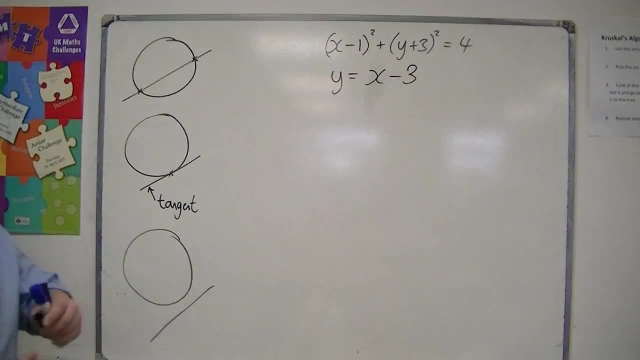 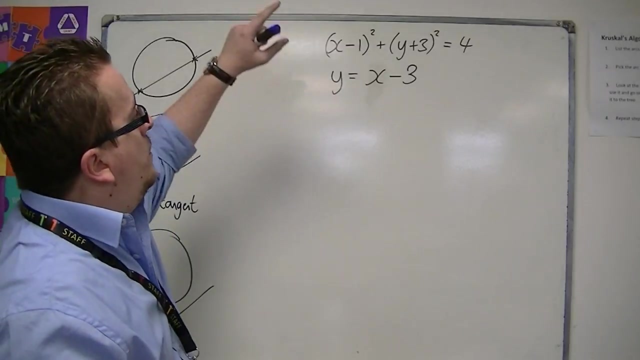 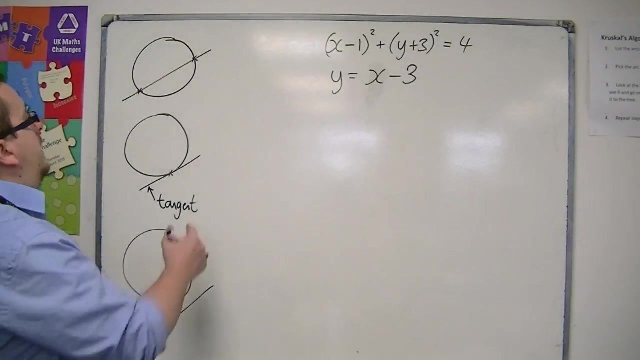 y. sorry, y is equal to x minus 3.. Okay, So we've got the equation of a circle and we've got the equation of a line, And we want to determine whether the circle and the line intersect or not. And if they do intersect, then whether we have two distinct points or 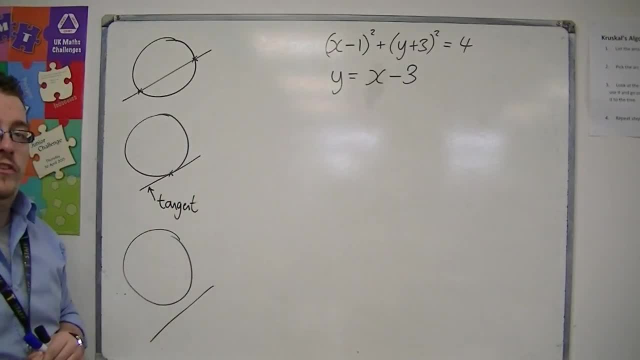 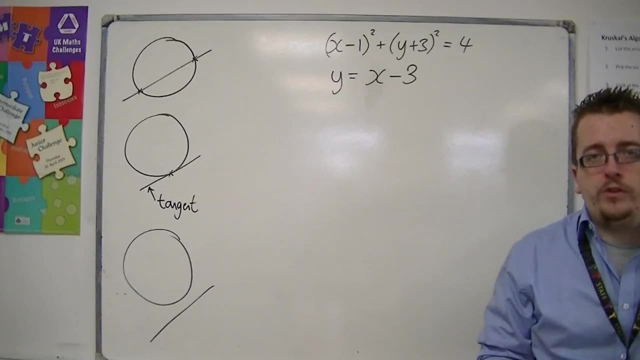 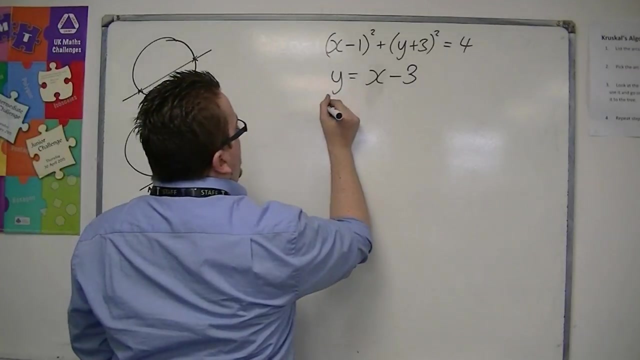 just the one, And so this line would then Therefore be a tangent to the curve. So whenever we deal with intersections, we use simultaneous equations, And so we substitute this equation into the equation for the circle, So we would have x minus 1 squared plus y. 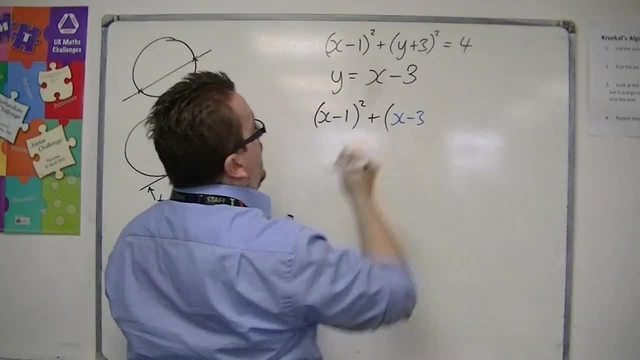 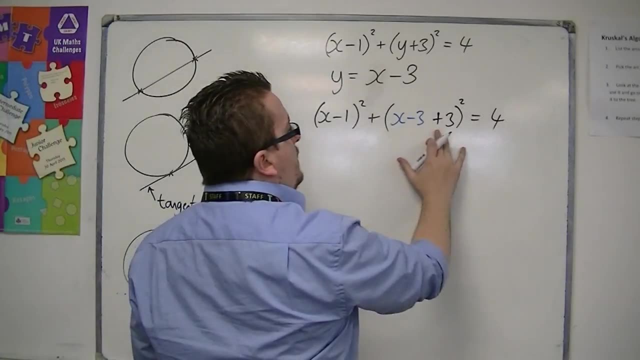 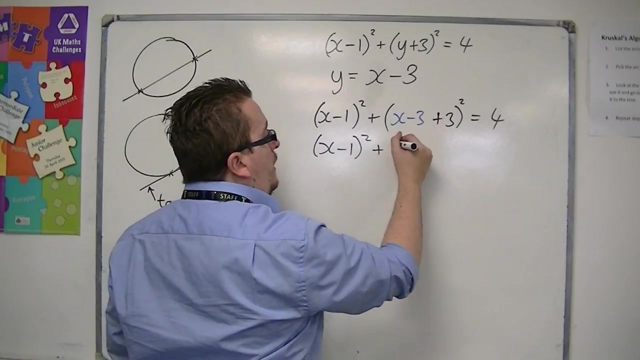 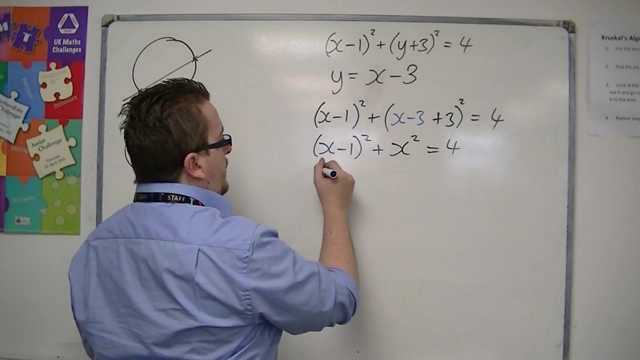 which is x minus 3, plus that 3 squared is equal to 4.. So let's simplify this bracket so that we get x minus 1 squared plus. well, that would just be now, because minus 3 plus 3 is 0, just x squared. So then multiply out the brackets. 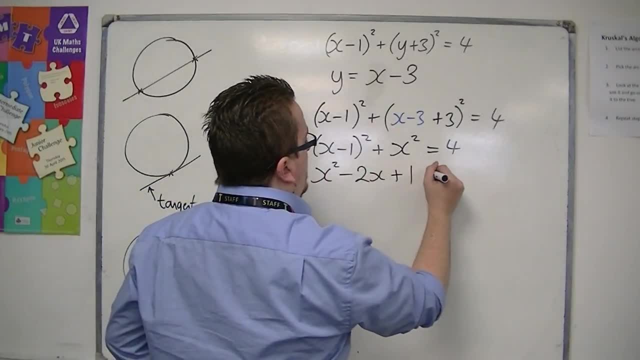 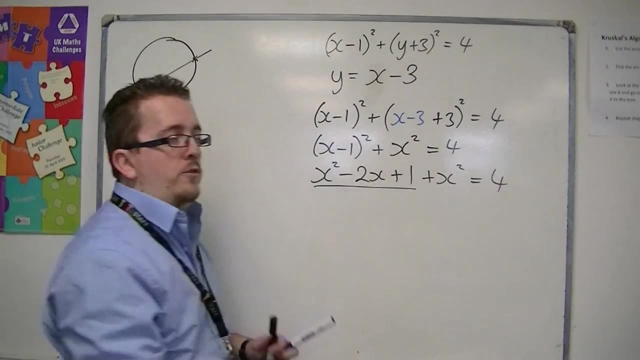 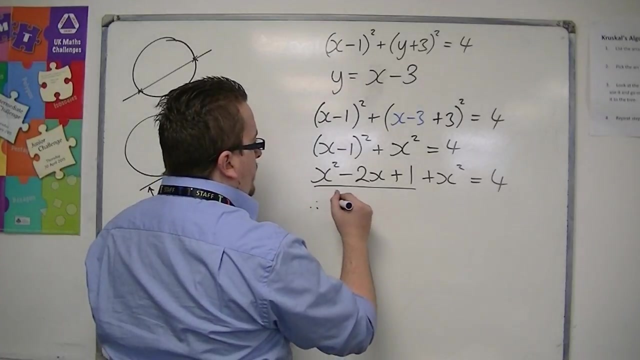 So we get x squared minus 2x plus 1 plus the x squared is equal to 4.. So that's been multiplying out the double bracket and that's the x squared from the last line, And then rearrange everything so we get everything onto the left-hand side. So we've got 2x squared. take away 2x and 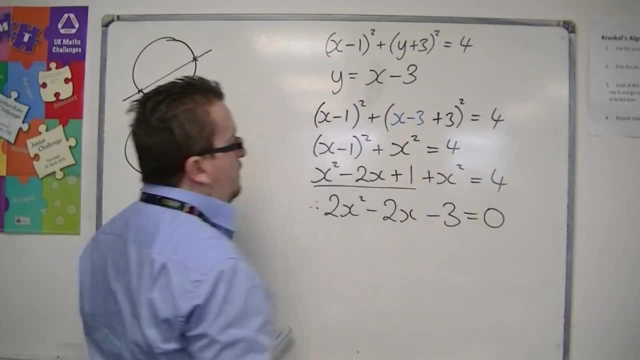 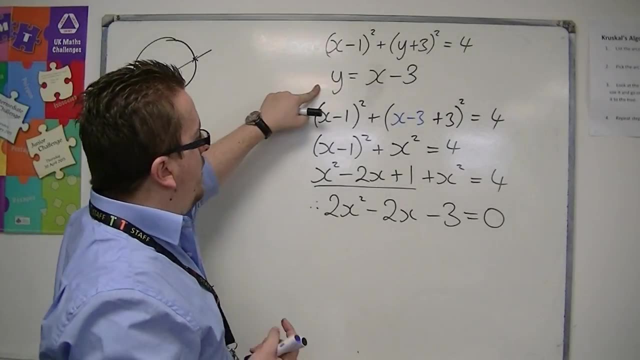 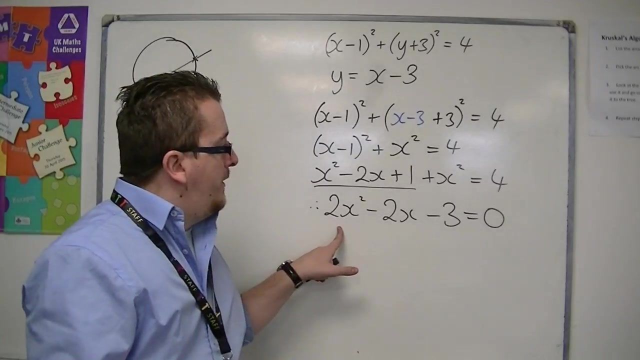 then take 4 from both sides will be minus 3, is 0.. So in working with the simultaneous equations of a circle and a straight line, we have ended up with a quadratic, And it is to do with this quadratic solving. it would allow us.